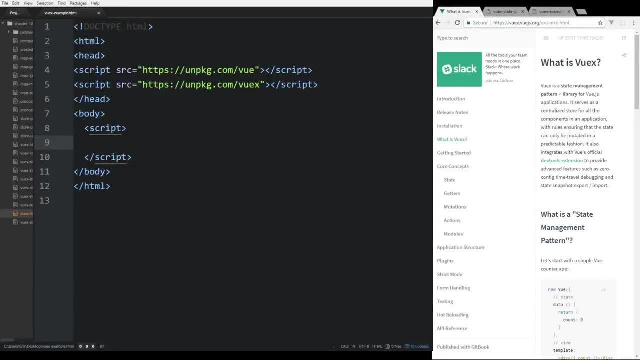 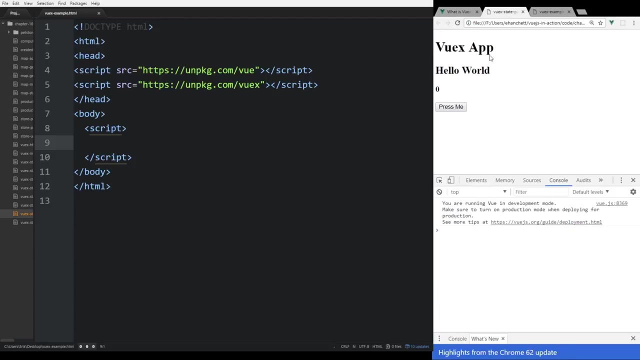 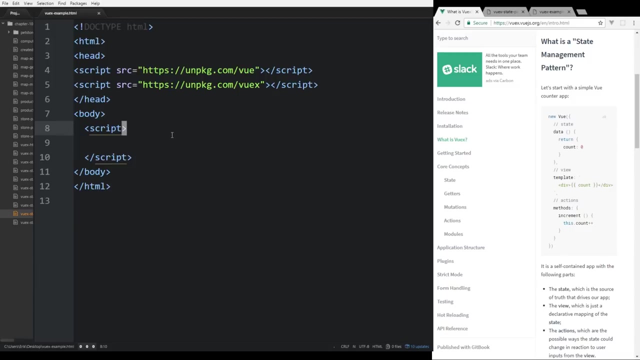 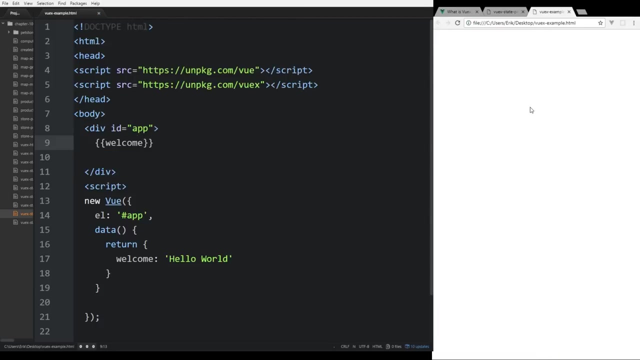 Hey guys, today we're going to look at Vuex. We're going to do it quickly in 10 minutes. So let's begin. So if you guys don't know, Vuex is a state management library pattern and library for Vue.js. So you may, if you're in the rack world, you may have heard of Redux. You may have heard of patterns called like Flux. So they're very similar. Both Vuex and Redux are kind of based on something called Flux, which is a type of pattern where we're dispatching actions. And we have different types of state. So we're going to go ahead and create just a really simple app. So if you can see right here, this is our app. We have a welcome message. We have some messages that are coming from our Vuex. And then we have a button that increments. So nothing too special here, but this is really important to us because we just want to learn some really basics of how this works. So let's go ahead and just create the basic part of our app here right now. So you can see here, I just went in and just copied and pasted some basic HTML code. I included script tag for both Vue and Vuex from a CDN here. So if we go new Vue. And then we'll call app. And we'll call, actually go EL. And then we'll call this app. And just to make sure things are working, we're going to have a data function here. It's going to return an object. And that object we're going to have one. Welcome. And welcome, we're going to put in hello world. And then inside here, of course, inside our body, we're going to have a div tag. We're going to have an ID equals app. And remember, you're always going to have to have at least one div tag in here for your Vue application. And then we're going to put in double brackets. And we're going to put in welcome. So we're just going to make sure this works. Refresh it. Okay, we see hello world. So we know we got that working. 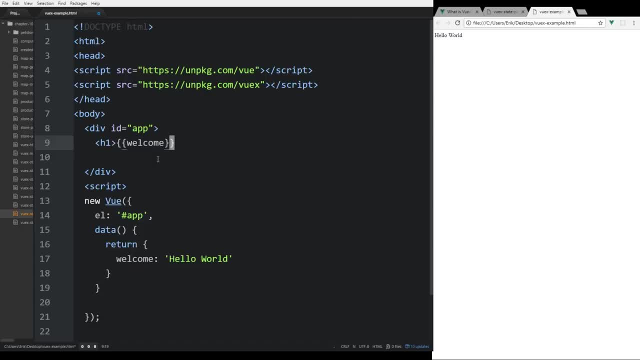 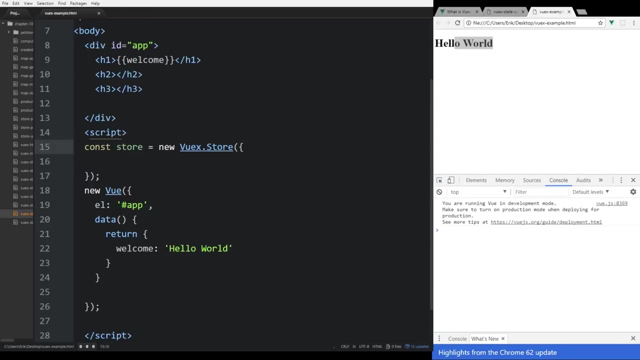 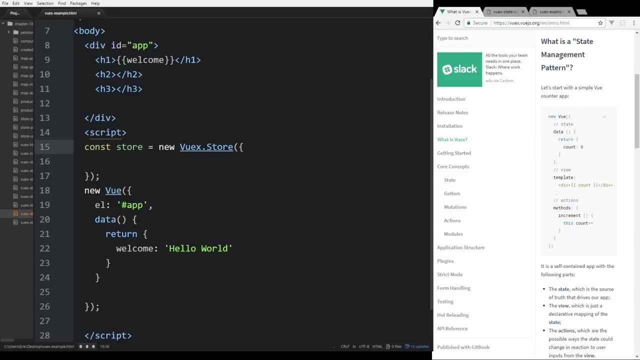 So let's just, let's do this. H, we'll put it in H1 tags. We're not going to do any CSS or anything in this. We're just going to do some really basic HTML. And then we're going to introduce Vuex here. So let's go ahead and create Vuex. Now, you guys are probably wondering, I'm actually using just a single HTML file here. But we could certainly do everything we're doing here using Vue CLI. So in a future episode, I'll go ahead and do a more advanced look at Vuex. And we'll go ahead and put it into a Vue CLI project. This actually works just as well. I mean, pretty much everything I'm doing here, you can do inside Vue CLI. So if you learn it using this way, it's the same thing, basically. So I'm going to do a const store. I'm going to have it new Vuex.store. And I'm going to refresh it. Okay, my hello world's big. And I'm going to go ahead and open up the inspector here to make sure if you have any errors that I can catch it before it gets too late. And then inside here, I'm going to create some ways, some part of Vuex. Now, like I said, Vuex is a way a state management pattern. So normally in Vue, and the reason you may want to use something like Vuex, especially if you have larger applications, is that you end up using a lot of props, and you end up passing a lot of data from one component to another. And there are things like 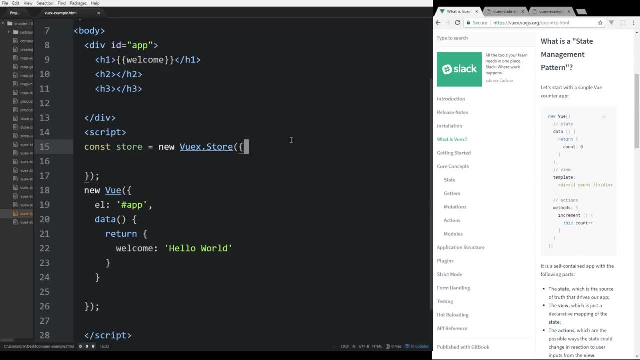 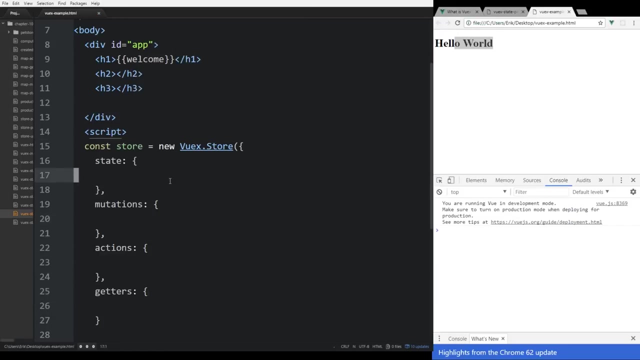 buses that you can create in Vue. But it really becomes pretty bloated after a while, and your data can be kind of stored in a lot of different places. So what the idea here is, with Vuex is that we're storing all the data in one central place, and any component can actually get it. So that is really important, because we don't want to have to, let's say we have a component, like we have component one here, and then it inherited it, component two is a child of component one, and then we have a child of component one, you know, child of child of component one, I mean, you can just keep on going, and you would have to actually pass everything from component one to child component one to child component one. And so the data can be all over the place. It's not perfect, and things can get complicated. Now, that's not to say you would put all your data, or all your, your, your state inside the store, you may actually be creating, you may actually have some local state and some of your Vue components. But some things that you may want to share between multiple things in your app you want to put in the store. So the first thing we do is there's four things we need to learn here in this 10 minutes, we're going to look at state, we're going to look at mutations, we're going to look at actions. And finally, we're going to look at getters. So these are the four that we care about. So in our state, this is where we're going to define kind of the data for our application that we want to store and, and, and have it be available throughout the application, and all our Vue.js instances and components. So let's just make right here, we'll create a message. We'll call welcome. Well, we'll call it. Yeah, let's call a message. And we'll put in Hello world. And then, well, 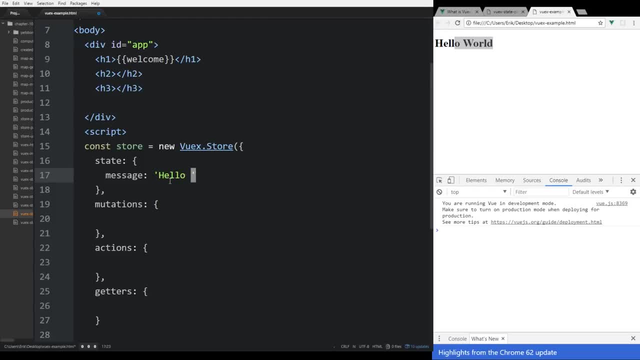 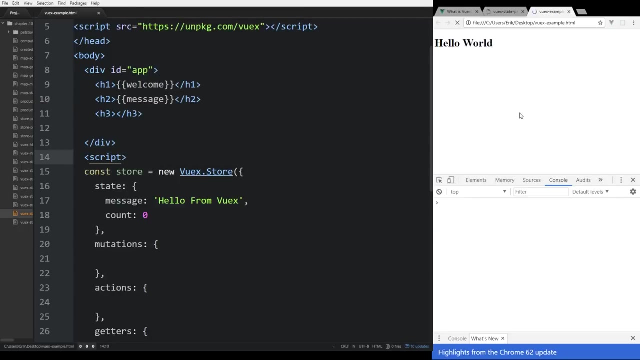 we'll put it a different message, we'll call it Hello from Vue.js. So we don't get confused. And then we'll put a counter, and we'll set it to zero. Now, if we want to access this message and count, there's a couple ways to do that. So first, if it's really simple, we actually getters are one way of retrieving information from our store, we can actually access it to without a getter. So we can do a computer property here. So we'll do computed here. And then I'll put a colon here. Make sure I'm doing this right. And then we'll name a computer property. So let's just call it, we can call it message doesn't can have the same name doesn't matter. And then in the message, we return it return it so we can return store dot state dot, and we call that message. And then inside here, we can grab message so let's see if that works all right so here's a hello from view x so you 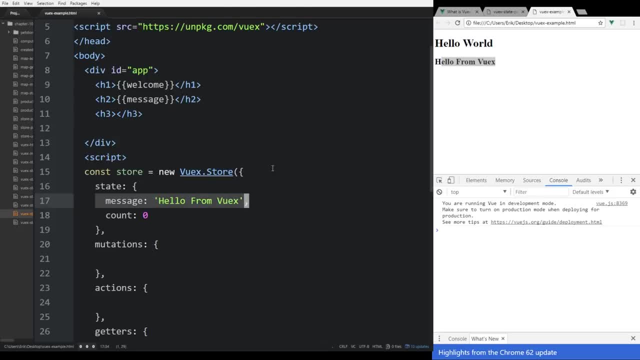 see here we're grabbing the information from our store and we're displaying it inside our h2 tag 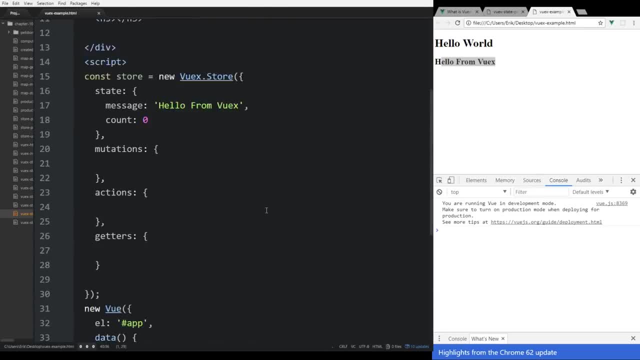 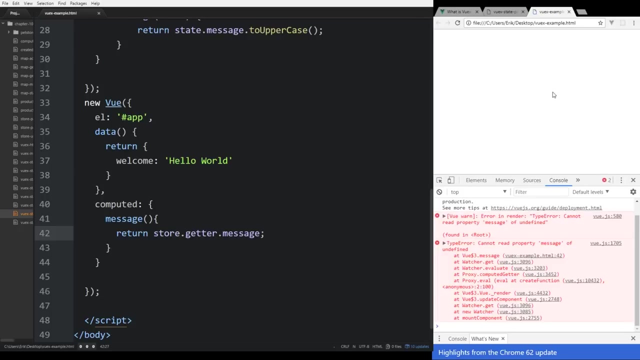 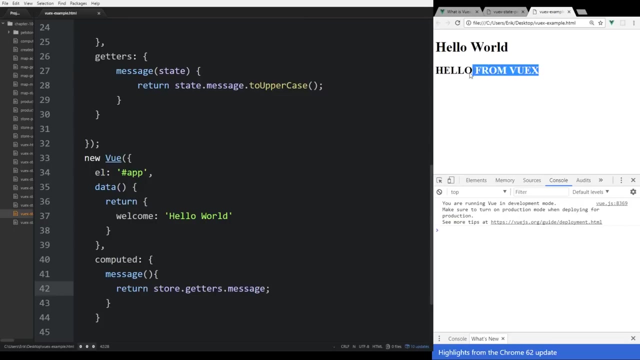 here by just using a computed property but let's say that you wanted to do you wanted your getter to let's say you wanted to make some kind of modification of this and instead of having a computed property and doing some modification to it here you can create a getter so every component gets it from the same place so this makes a lot of sense in larger apps so we can do this we can put in the getter we can call it message here and it actually takes a couple variables it takes a state well it takes one argument state and then we can return state dot message which is the name of our it our variable here message and then we can do something like two upper case something like that and then instead of doing restore dot state dot message we can do store dot getter dot message so we save it there and message of undefined so let me make sure i got this right getters and i'm missing an s so okay you can see here it's all capital letters hello from view x i'll make that bigger so hello from view x and we know it's working so now instead of getting it directly from the state we're getting it from the getters so you can see you can imagine that you can set up a bunch of different getters here and do a bunch of different things and have all your components grab it and you're not going to have to you know repeat the 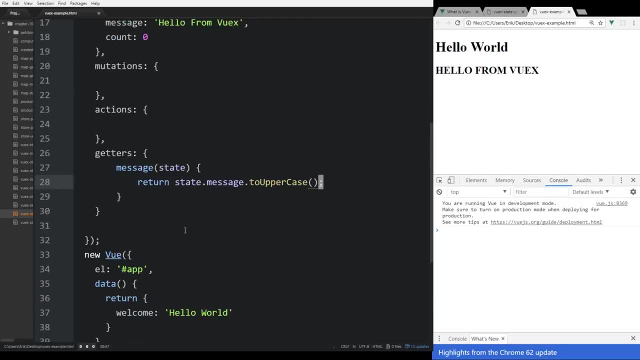 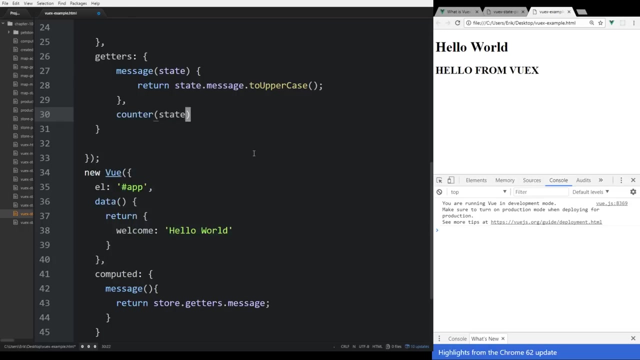 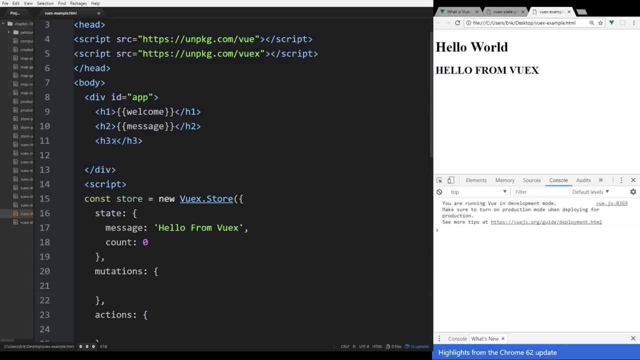 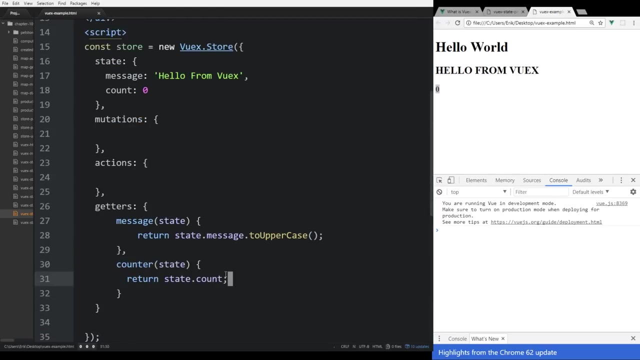 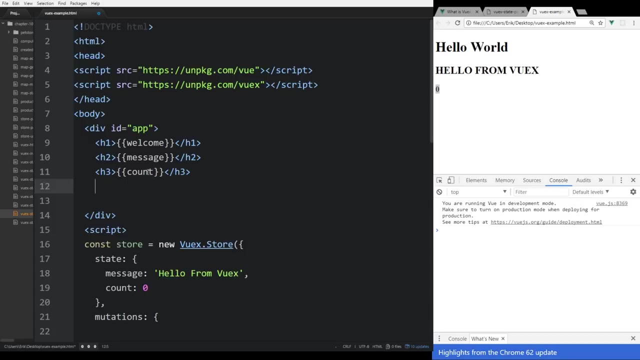 same code in every single component so that's one way to doing it so another thing we can do is mutations so let's take a look at our counter here so let's go ahead we can do another computed property and let's create another getter so we'll call it counter once again it has an argument state and we can return state dot count and then inside here our computer property we can also do the same thing here we can have a count and then it can return store dot getters dot count so if we refresh it and we use the name counter and we called it here we'll put in count there it is so you can see zero here so we're getting it from the getter and then we can return store dot getters dot count and then we can from this computed property it's returning it out of here just the state dot count but what if what if we wanted to do some kind of mutation on this and change it so let's create a button here and we'll just do a button we're gonna have a click action attached to it we're gonna call it pressed and we're gonna call it I'll call it increment counter and if we save it we have increment counter of course we're 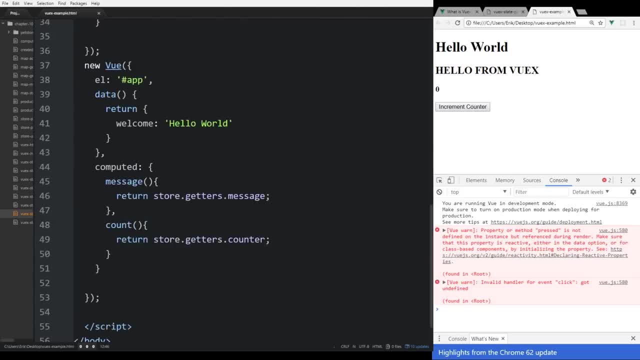 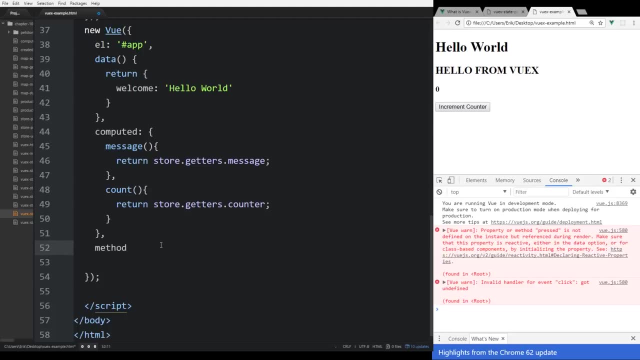 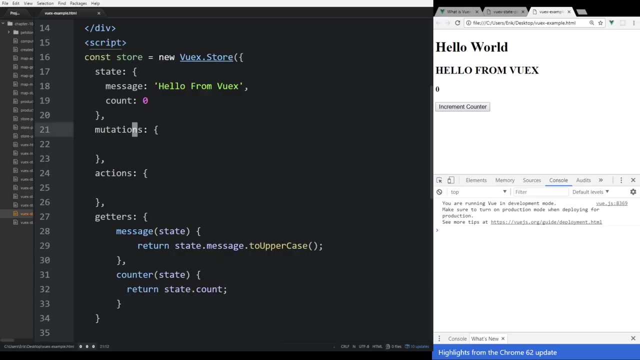 gonna get an error because we haven't created this action yet but let's create it so we'll go back down here right after computed we're gonna create something called method I think it's methods it's an s and that's gonna be an object and then we're gonna have our pressed and then in our pressed we're gonna do something so let's save it all right so we no longer have it but this breast doesn't do anything so what we can do now is we can create our cut � 연습 can have a mutation in here. So let's create a mutation that increments the counter. So we're going to call it increment. And we're almost up out of the 10 minutes. So this can be a few minutes after 10, but that's okay. We're going to have a state on it and a payload. And then in the state and payload, we're going to do state.count. And then we're going to plus equal the payload. So what this is saying is every time you do the increment, it's going to take the state. It's going to take something you pass into it and then equal it, add it to it. So then what we could do here is we can do instead of getting it, we can do this. We can do store. 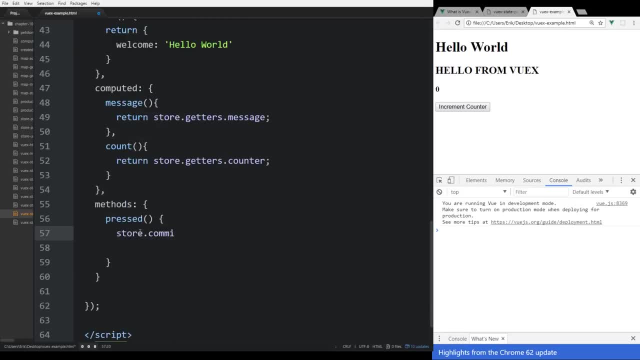 And we use something called commit. And we do commit. And then we can call the name of the mutation, which we call the increment. And we can add 10 to it. So let's try that. 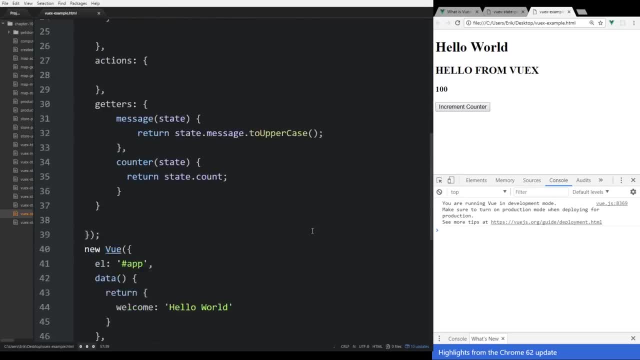 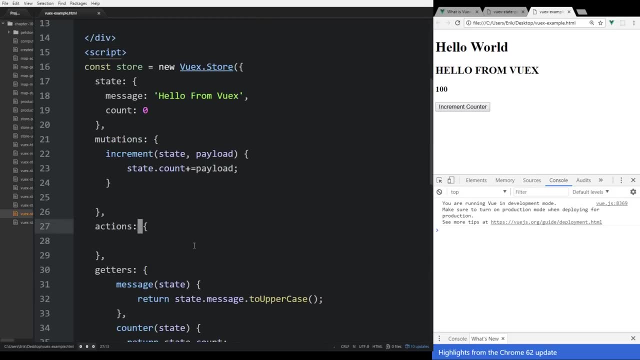 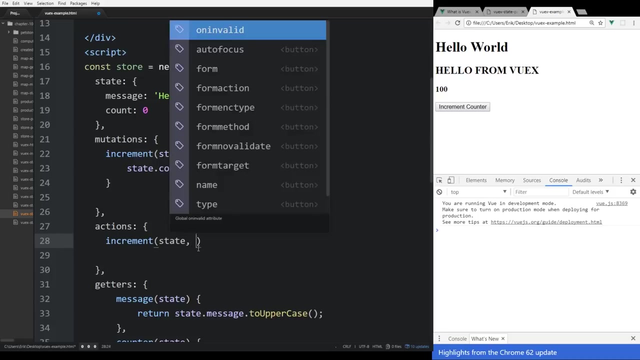 Okay, that works. So basically, we've reproduced what we had before. But really, really, really quickly, I know we're over our 10 minute allotment. We're going on to 11 minutes. But we really quickly, if you go to actions here, we can have an action called increment as well. And then inside the action here, we can put inside a state and a payload as well. And then inside the action, we can do state.dispatch. And then we put in the name increment. And then we put in payload. Now the reason we have actions is because you can actually access the mutations. 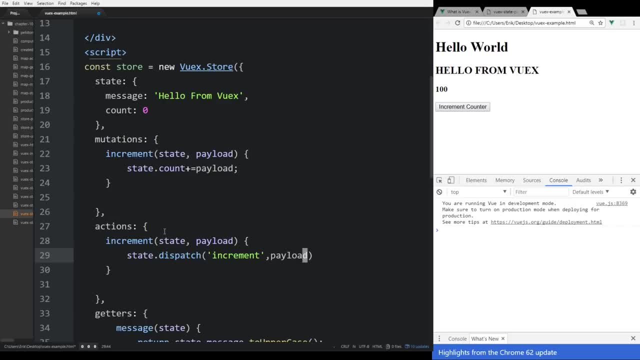 correctly but if you have something that's asynchronous then you must use actions mutations are always synchronous so this is always synchronous and actions can be asynchronous or